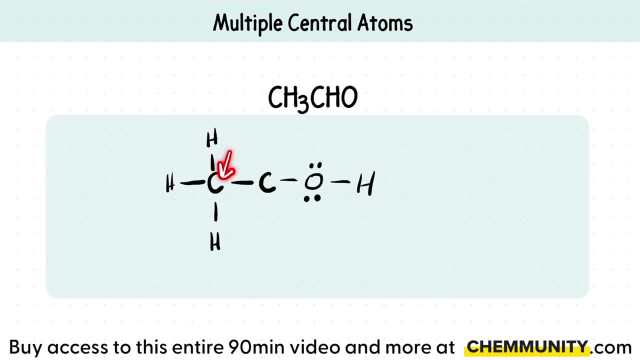 So this carbon is following it because it has four bonds, but this carbon is not. There's only two bonds, so there's only four valence electrons. So this doesn't follow the octet rule. This structure would be incorrect. because of that reason I can't say that the OH, that oxygen. 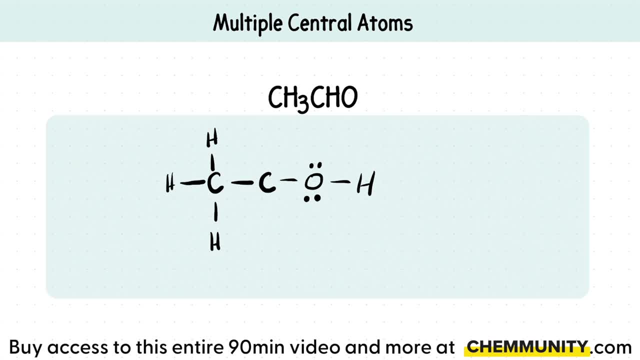 is bonded to hydrogen. Instead, we're going to do this a little bit differently and I'm instead going to say: okay, maybe it's just the oxygen that is bonded to that carbon and hydrogen is also bonded to that carbon, And that would be correct. Whenever you see this CHO, that is. 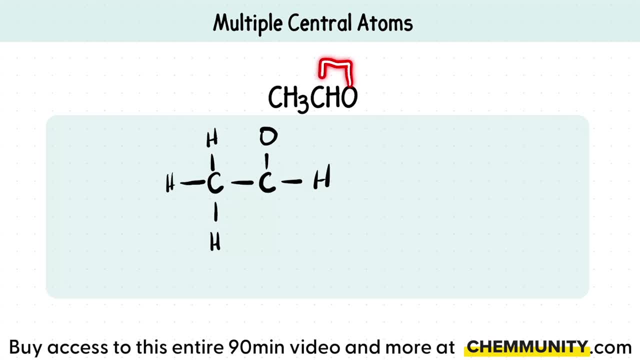 actually C-H-O. So we're saying that this oxygen is bonded to the carbon and this hydrogen is bonded to the carbon. Oxygen and hydrogen are not bonded to each other. That's only when you see OH, That's when they're bonded to each other. Now we're not done yet. Carbon still doesn't follow that octet. 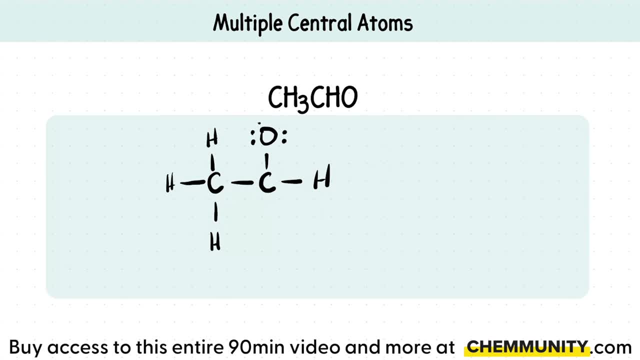 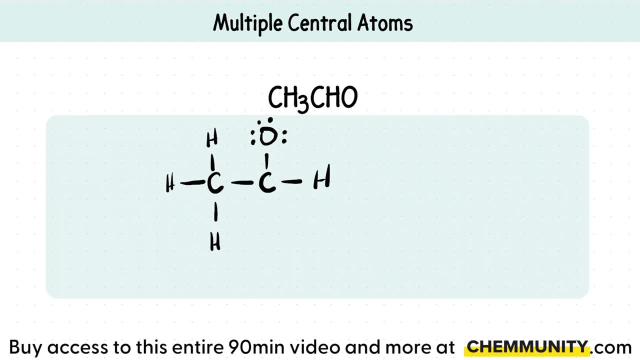 lone pairs, I chose to form that double bond. So as long as I erase one of them and form that double bond, that's fine. Also, it doesn't matter if I decided to place this double bonded oxygen on the bottom, As long as there's only one. typically you will see it on the top. but 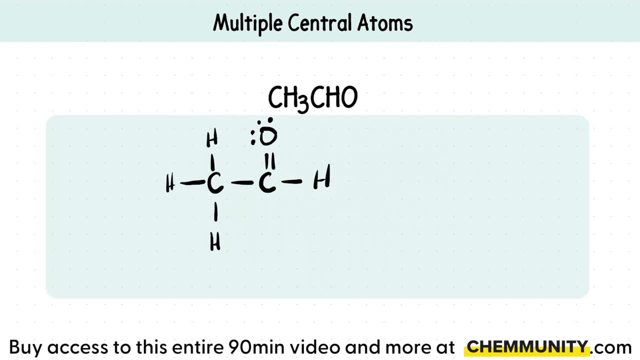 we're going to be moving it around as we go throughout organic chemistry, But this would be the correct structure. I know that because everything follows the octet rule- that it should right. This carbon now has four bonds, or a total of eight balanced electrons. Here's two, four. 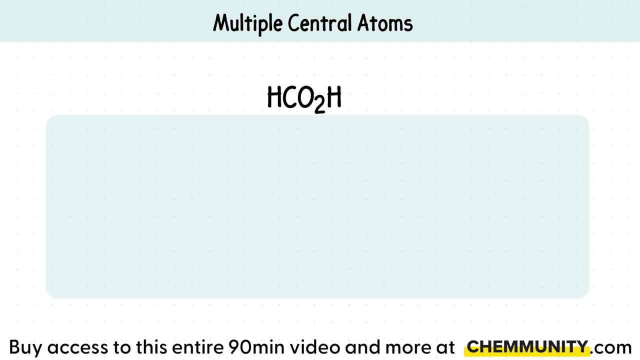 six and eight, Moving on to the next part. So this next one can also look a little bit different. So you could either see this sort of chemical formula look like this, or it could say H-C-O-O-H, Since this is just the 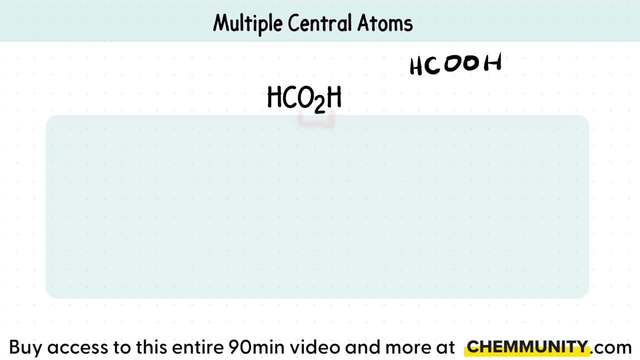 example, I'm going to say H-C-O-O-H. So this is just the example. I'm going to say H-C-O-O-H. So this is just the example. I'm going to say H-C-O-O-H. And there's a clue for you. right there We see O-H. So I know that oxygen will be bonded to. 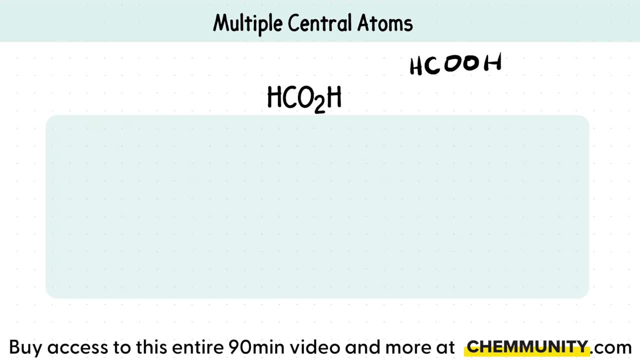 hydrogen. So, starting this off, this is already kind of telling me how things will be bonded somewhat. So if we were to just draw this all out, there's carbon, they're all bonded to each other- And if we left it here, let's see if this would be correct. First off, I know that our oxygens 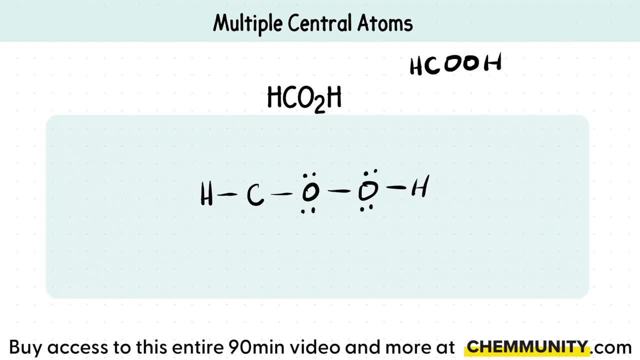 need to have these lone pairs- And that's something I want you to get used to- is if you were to see, let's say, oxygen just single, bonded to something that would then look like this, where it has three lone pairs. If oxygen is bonded to two different things, then that has two lone. 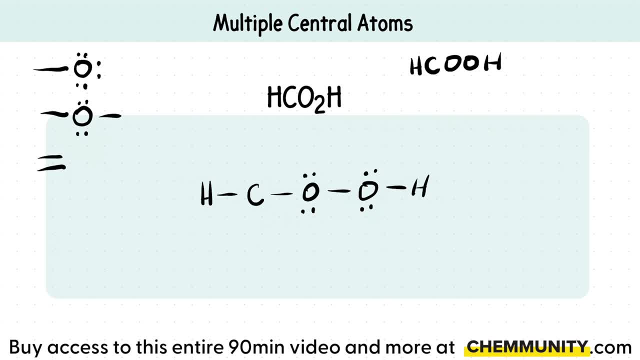 pairs. If oxygen is double bonded, then and it's on its own, as we saw before, that also has two lone pairs and so on. So that's something that I want you to get comfortable with And just quickly be able to spot how many lone pairs will be on oxygen, nitrogen, sulfur and so on. 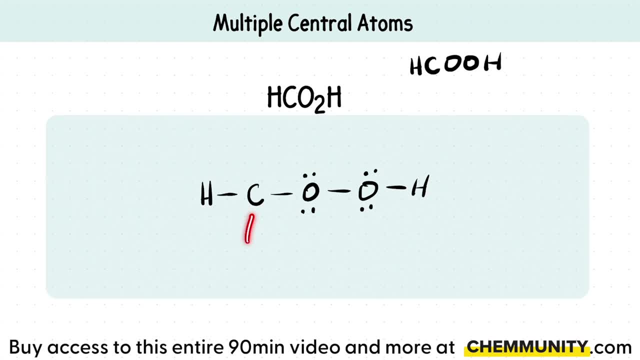 Okay. so going back to this, carbon is not happy because it's not following the octet rule right now And it needs to. Let's see if I were to place, maybe move this and make a double bond. let's see if that'll make it happy. So move this. that's now a double bond. Well, we only have two. 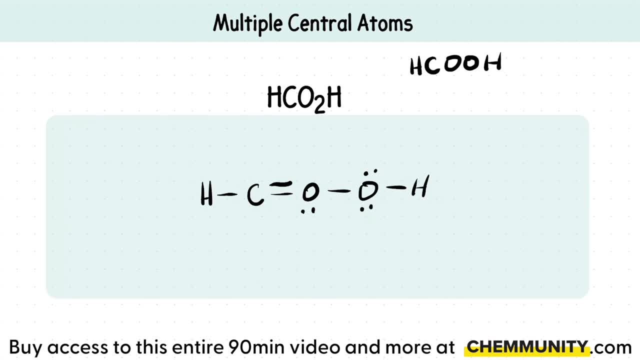 six electrons. Nope, still not happy. Okay, what if I were to move these electrons as well and then form a triple bond? Let's try it. If this moves and that now forms a triple bond, well, carbon is technically happy because it does have a full octet, This oxygen. 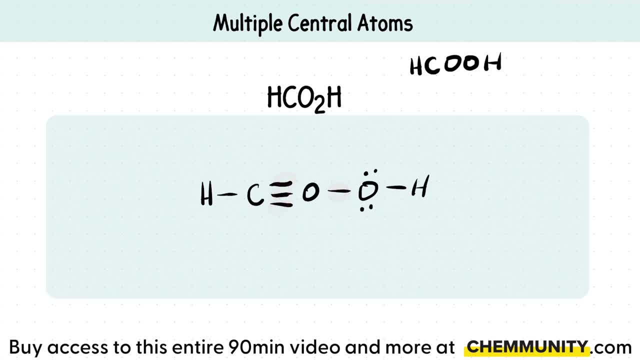 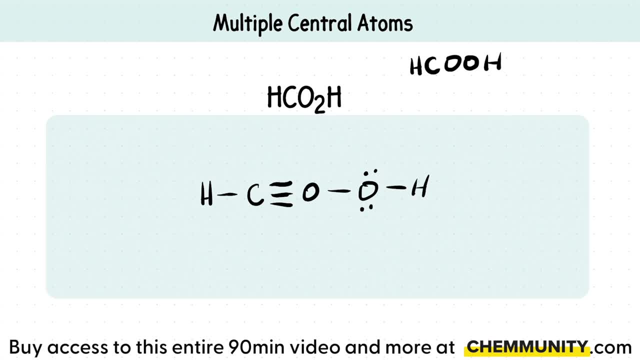 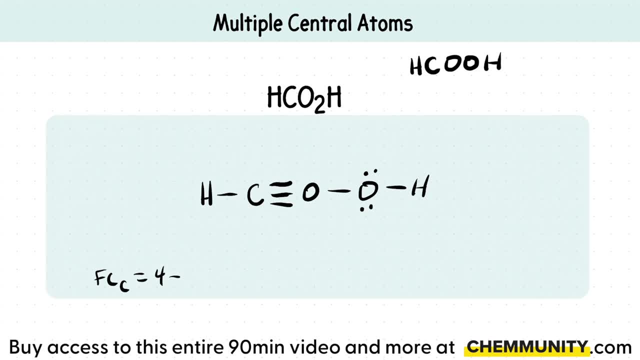 we know our valence electrons are four. I'll subtract that by how many actual electrons are currently bonded. So there's one, two, three, four and that's zero. Okay, that's happy. Next I'll do the next, oxygen that is next to that carbon. So formal charge of oxygen, I know. 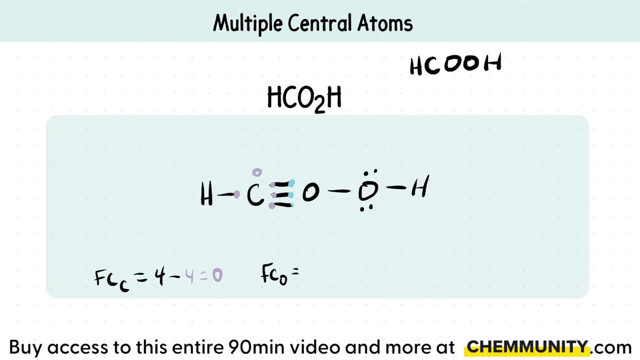 let's see how many bonding we have. There's one, two, three, four, So there's four. Let's start off with six valence electrons minus the four electrons on that oxygen, So that's a positive two, Positive two. Okay, I'm going to stop right there, And the reason why I would stop right there is: 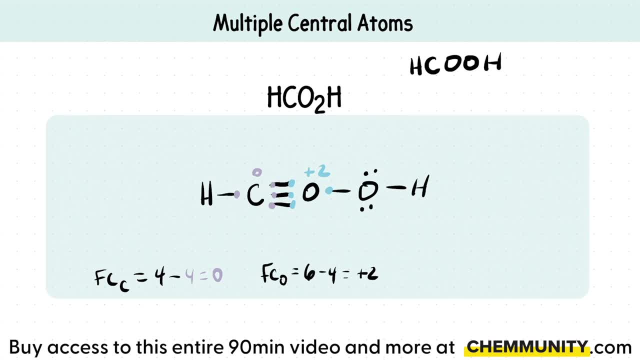 because, remember, our guidelines stated that the most electronegative element wants to either be zero, if it can be, or negative. It did not say it wanted to be positive, And our most electronegative atom is oxygen. However, if that's positive, that's incorrect, It's not going to be. 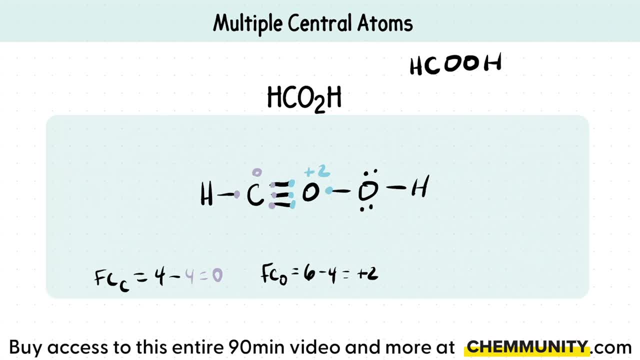 stable, And that's telling us. you know what The structure is incorrect. We can redraw this a different way, And that's exactly true. This is not how we would draw this out. We would not actually place everything laid out. So I'm going to erase this and I'm going to show you. 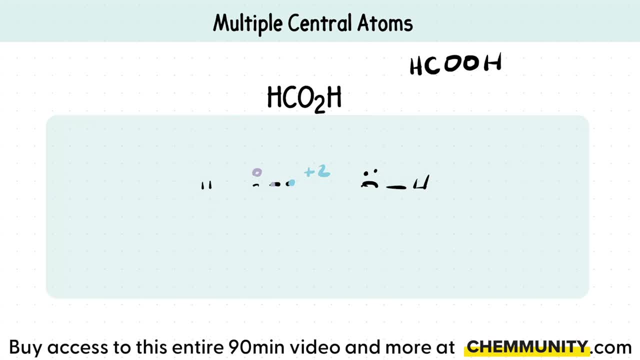 how this would look. This is another one that I want you to get familiar with, And it's specifically when we start to see this part. So COOH, or it can be written this way, So I'll start off with just carbon again, and that's still bonded to hydrogen. There's nothing. 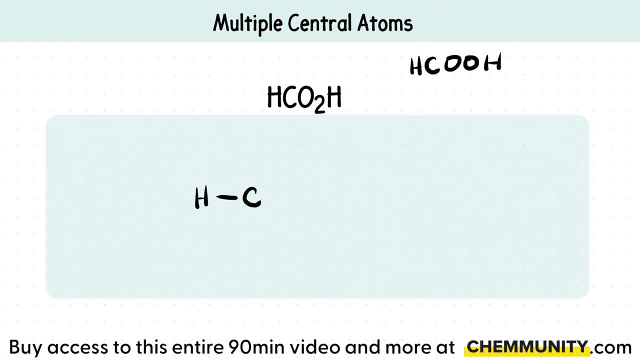 wrong with that. The places where it was wrong- was just how oxygens were bonded. They're not bonded, they're only bonded to carbon. So I only have one oxygen here, one oxygen here, and then that's bonded to the hydrogen, since I saw that OH at the end. So that's that OH at the end. Okay, Now I'm. 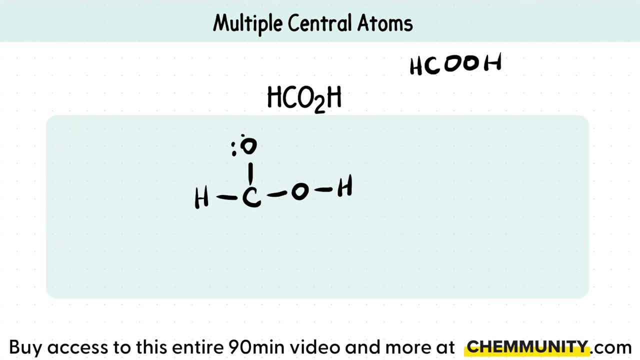 going to place all of the electrons. So there's two, four, six and there's only two lone pairs Carbon. again, it needs a full octet. So what I'm going to do is I'm going to start off here. 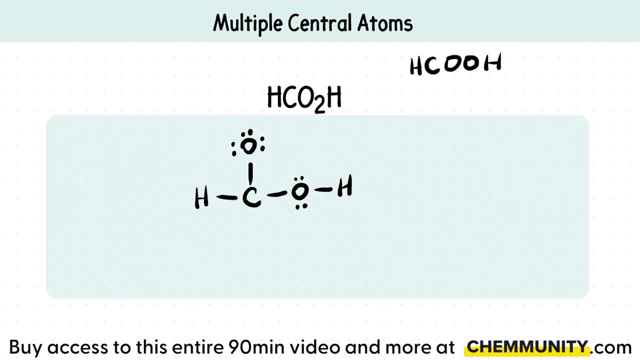 So I'll start off here. And the reason why I know to automatically start changing this structure or forming a double bond here instead of this one is because of the formal charges. So I'm going to find the formal charge of this top one first. 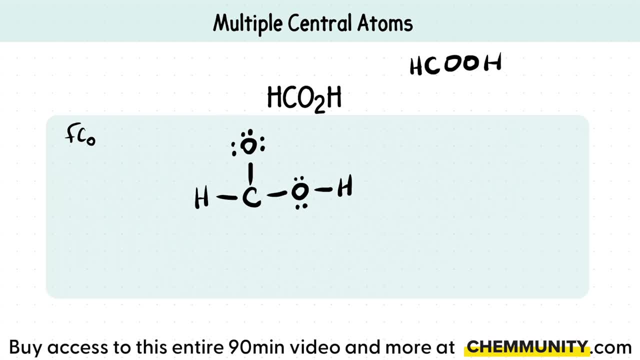 So formal charges of oxygen. I'm going to say one, That's valence. electrons is six minus however many electrons it currently has. So that's one, two, three, four, five, six and seven. This has a negative one formal charge. I'll do the formal charge for the second oxygen now. 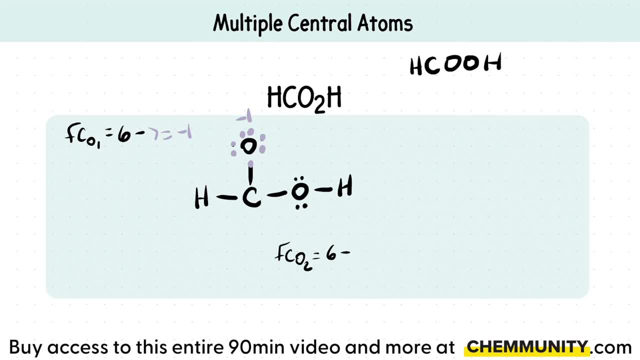 So that's six valence electrons minus however many we actually have. So one, two, three, four, five and six. That has a formal charge of zero. Which one is most preferred? The neutral formal charge. So because that has a formal charge of zero, I know that I'm going to leave it alone. 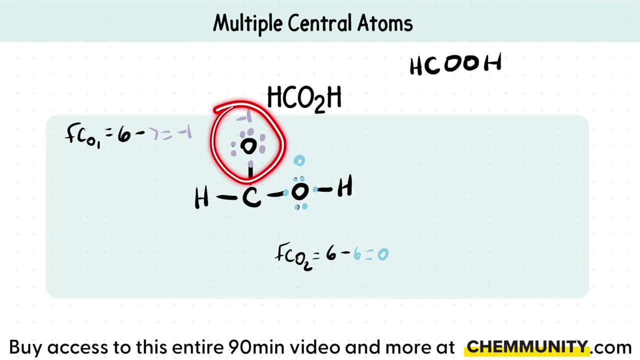 So I want to touch that. It's happy. Instead, I want to change this negative one to potentially be zero, And that's exactly what you're doing there. When you're moving these electrons, a lone pair, to form a double bond, you're going to have a formal charge of zero, So that makes it even. 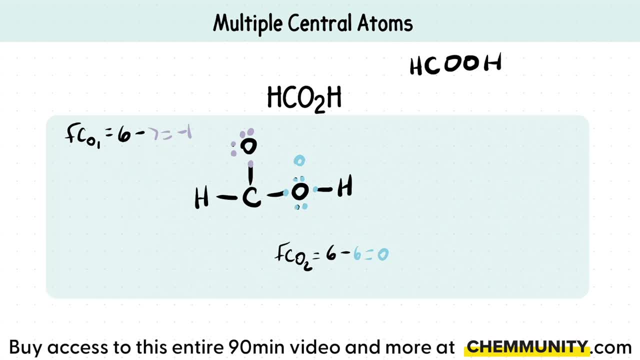 more stable. So let's move this lone pair and form this as a double bond. That would be the correct structure, So let's erase this. So something to know for your formal charges, since before you start a double bond, you're going to have a formal charge of zero, So let's erase this. 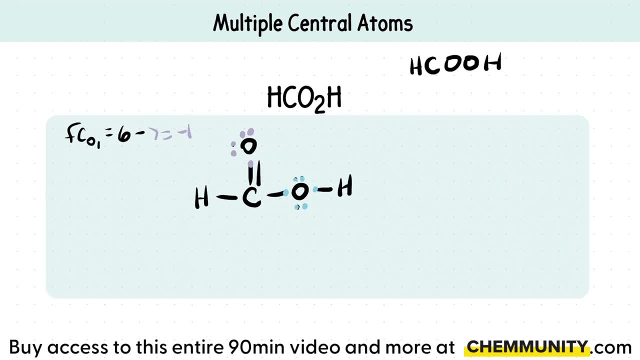 Before I showed you how the bonding is and how many lone pairs there would be, I want you to get familiar with the formal charges and how you can quickly see that as well. This has a formal charge of zero. Same with a double bonded oxygen with two lone pairs. That has a formal charge of zero. 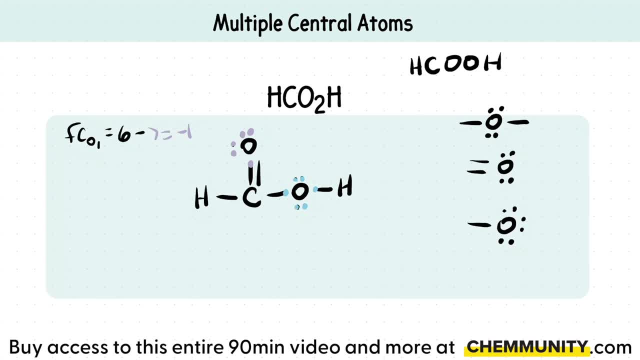 Our single bonded oxygen with three lone pairs has a formal charge of negative one. So this would be negative one. formal charge of zero. formal charge of zero. This one should make sense that they both have a formal charge of zero, because there's two bonds here And then this is a double. 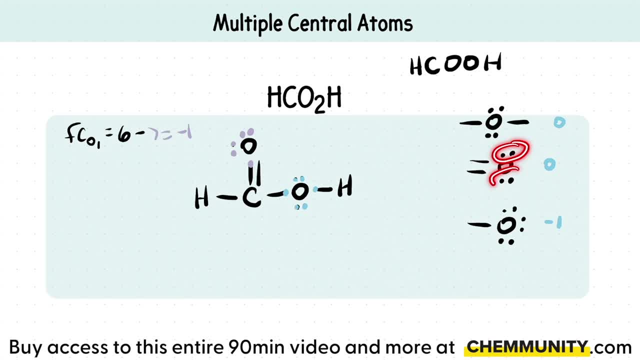 bond. There's two lone pairs. There's two lone pairs here, Okay, So I want you to start getting quick at this and just being able to quickly find and spot the formal charges. Eventually, when you do enough of these, you just tend to remember what the formal charges would be, since. 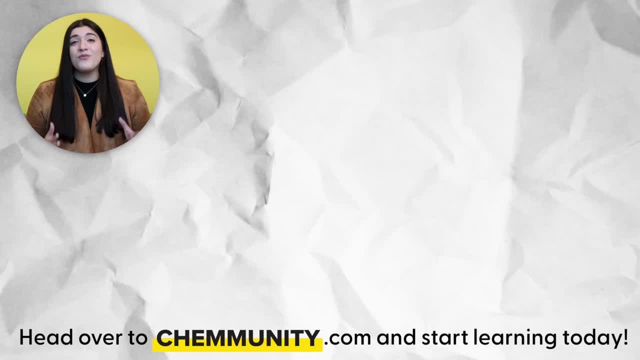 you see this so often. All right, let's do this next one. I have more videos, just like this one on communitycom. Thank you,